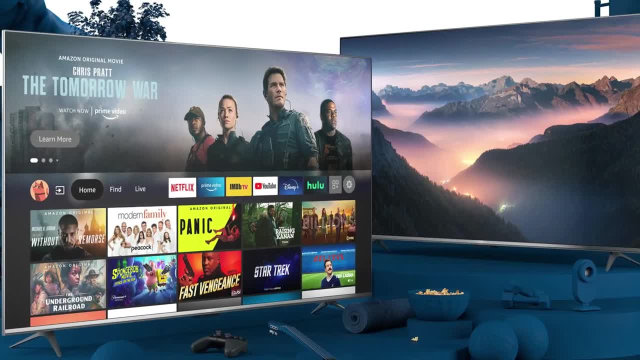 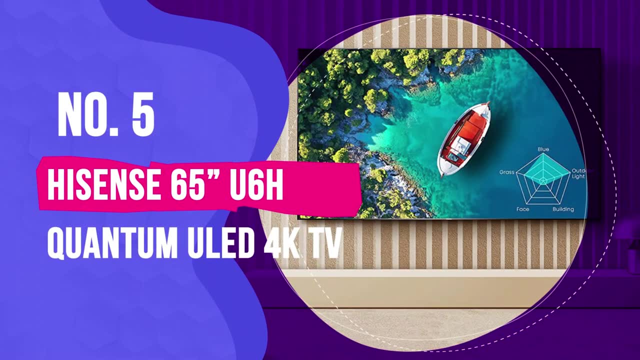 on the TV with AirPlay for more ways to show photos, videos and stream music. Number 5. Hisense 65-Inch U6H Quantum ULED 4K TV. Last year's Hisense U6G stood out for hitting the pinpoint sweet spot between performance. 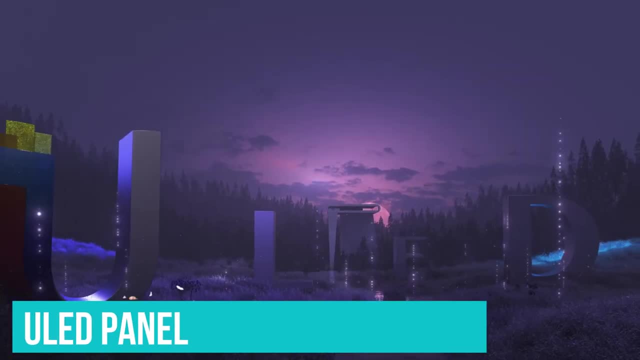 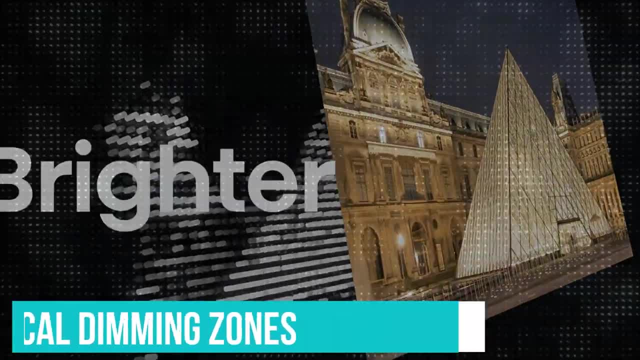 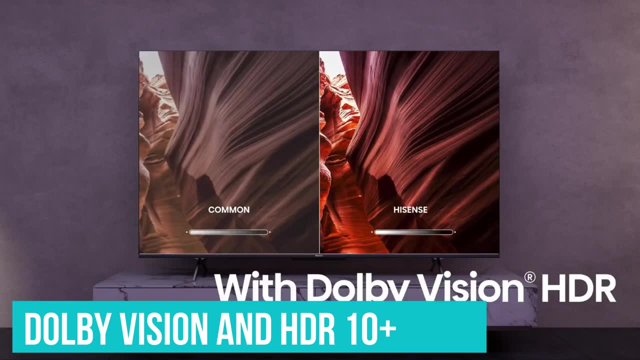 high-definition, high-definition, high-definition, high-definition, high-definition, high-definition. array, local dimming, 48 local dimming zones and up to 600 nits of peak brightness. Combined with support for HDR formats that include Dolby Vision and HDR10+, the U6H has plenty of tools at its 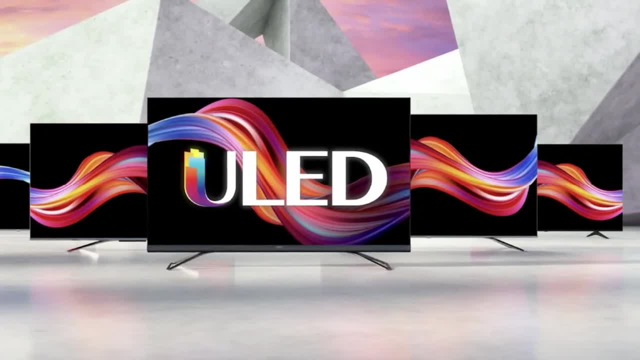 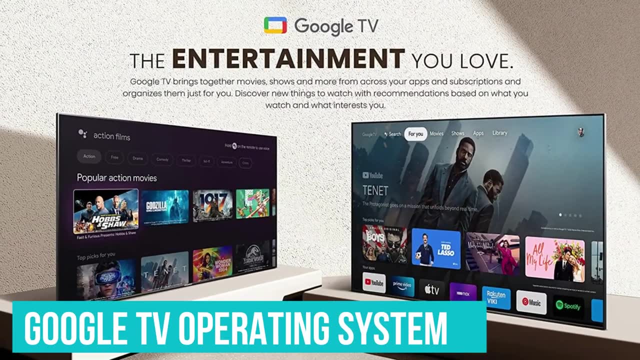 disposal to deliver an incredibly detailed picture for a price that won't break the bank. Hisense isn't done, however. The U6H marks Hisense's transition to the Google TV operating system, and their display offers gaming-friendly features like a variable refresh rate of 60Hz. 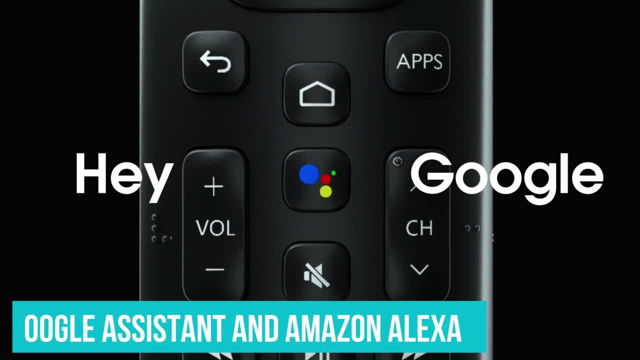 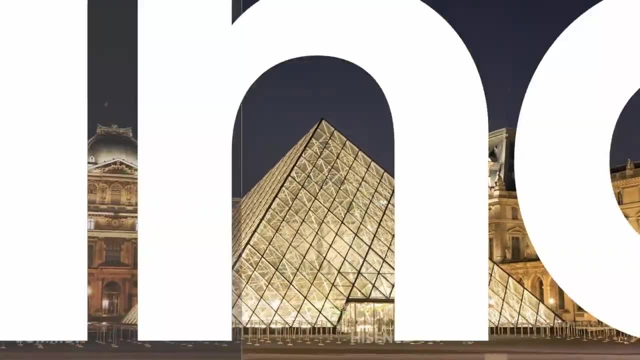 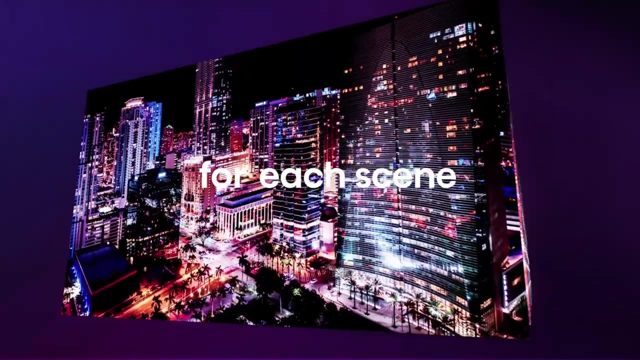 It also offers both Google Assistant and Amazon Alexa and supports Dolby Atmos to help make the sound as immersive as the display. Perhaps the U6H's most intriguing component is its processor, called the HiView Engine 4K. The processor acts as the brains of the entire ensemble, automatically adjusting the picture in real time for the best quality. 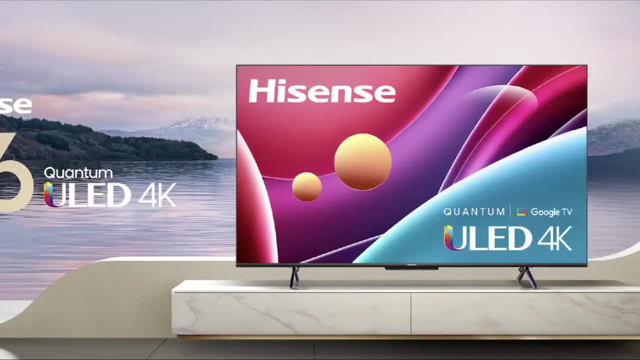 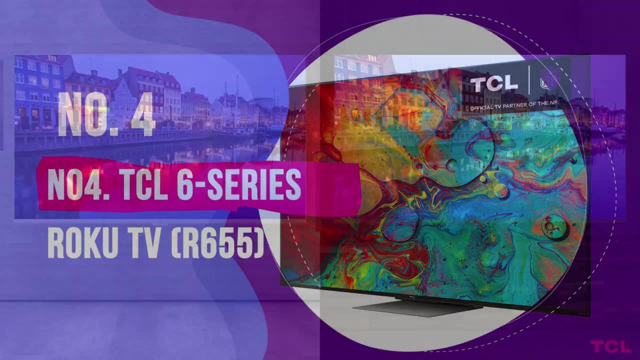 Altogether. it's a wildly capable 4K TV for a ridiculously inviting price tag- Number 4.. TCL 6-Series Roku TV R655. TCL has long been acclaimed for bringing a lot of performance to TVs that don't cost a lot of money. 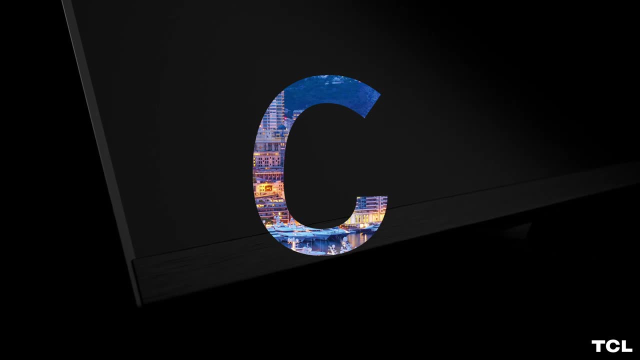 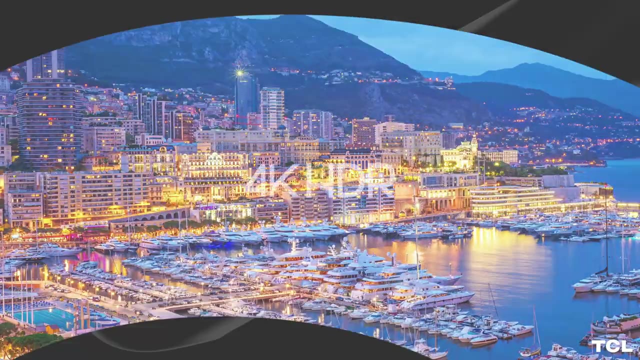 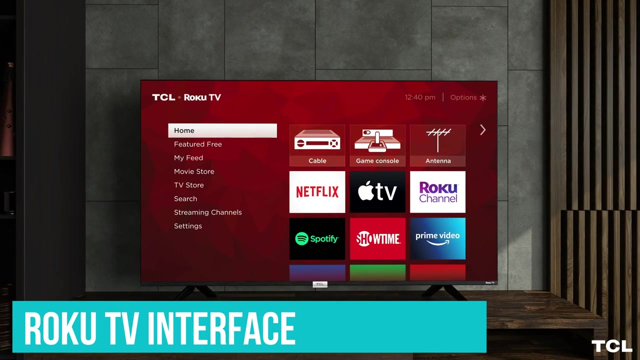 That trend continues with its latest 6-Series Roku TV, the 65R655,, which amps up key aspects of its performance, particularly brightness and gaming potential, while keeping the price at $999.99.. Throw in super easy-to-use Roku TV interface. 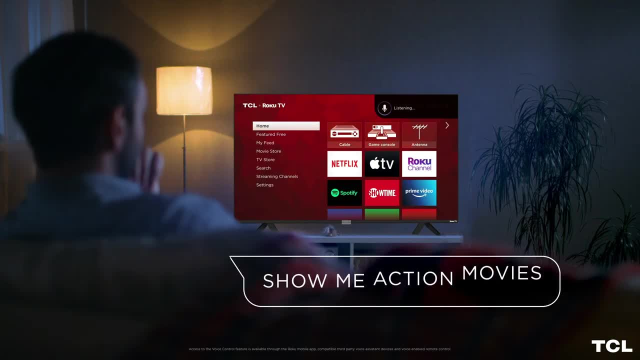 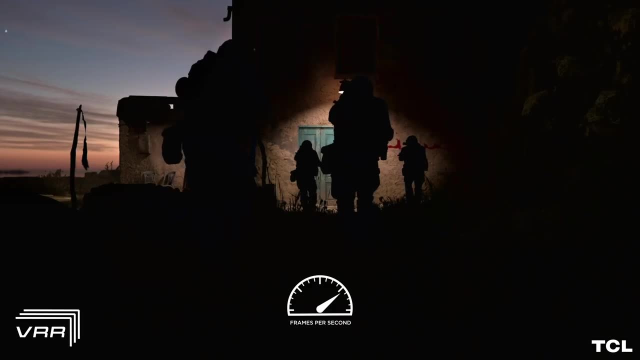 and you have the best performance in the world. You have a set that more than delivers on its picture promise without busting your budget. If you're a gamer or you can't bear to give up bright and dark details when watching movies or TV shows, you'll find a lot of love about it. 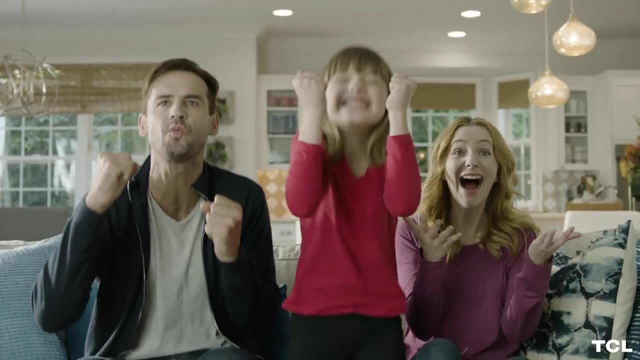 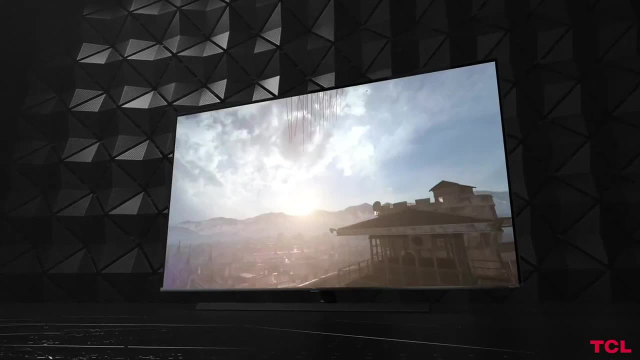 Its sound and color performance can't match the top TVs on our list, but they can't stop this set from punching well above its weight where it counts. So if maximizing your TV buying color is your goal, Roku TV is a small price to pay for a TV that's as packed and as low-priced as the TCL. 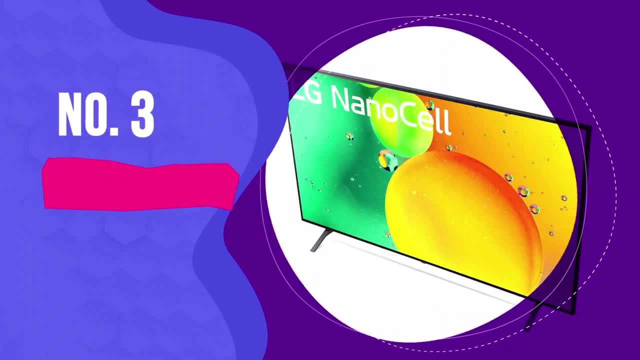 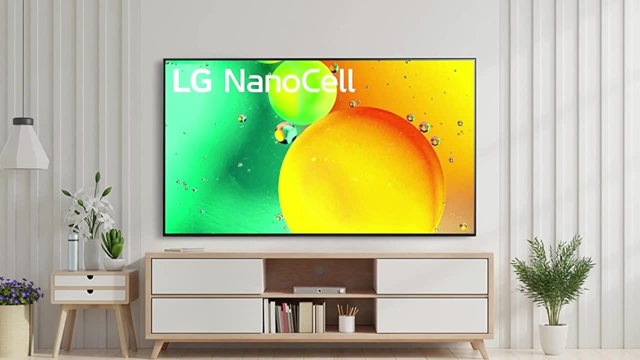 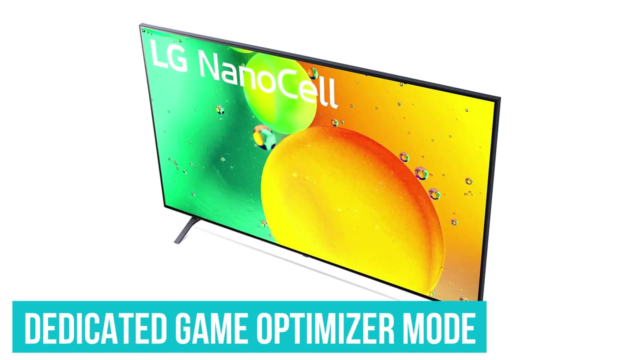 The TCL 65R655.. Number 3. LG Nano 75- 55-inch Console. gamers looking to save a bit of cash on a new TV for their gaming space should definitely consider the 55-inch LG Nano 75.. This TV has a dedicated game optimizer mode and dashboard. 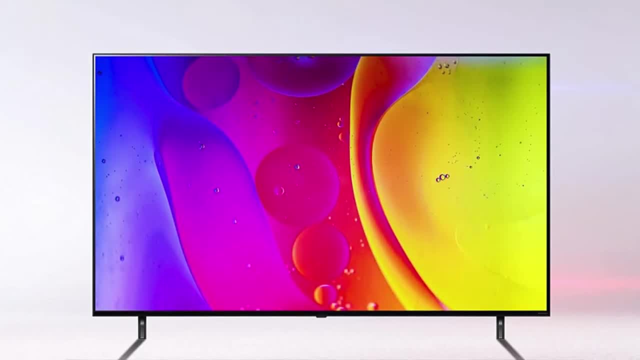 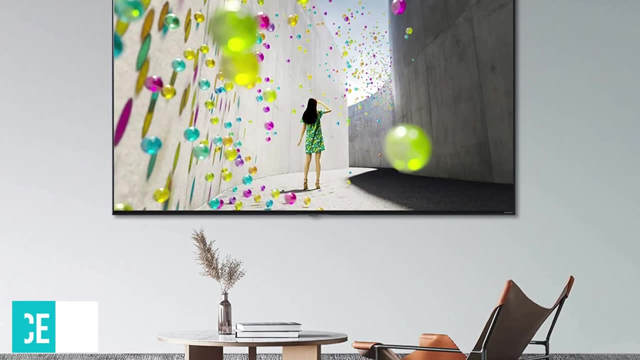 that lets you monitor things like frame rate, latency and contrast, so you can fix issues before they can ruin your gaming session. It also supports cloud gaming via Nvidia GeForce Now, so you can play your favorite games or your favorite PC games from the comfort of your couch. 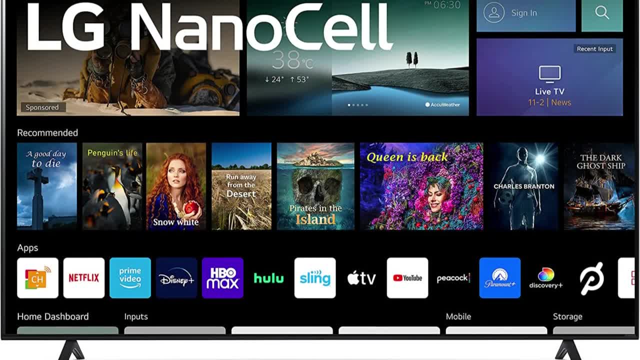 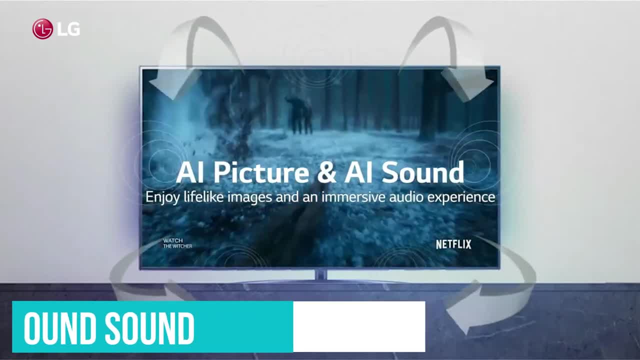 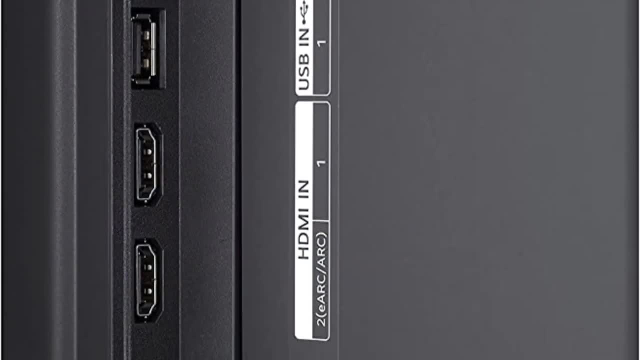 You can also create a custom audio setup by connecting soundbars, subwoofers and speakers to the TV via Bluetooth, Or you can enjoy virtual 5.1CH surround sound via the AI-enhanced built-in speakers, And with three HDMI inputs you can connect multiple consoles at once. 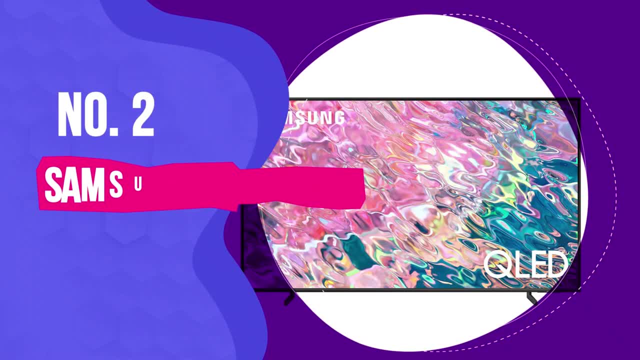 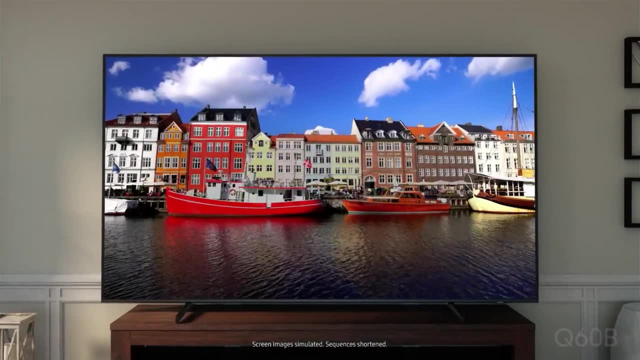 and switch between them on the fly. Number 2. Samsung Q60B 50-inch. If you're in the market for a new TV but don't want to break the bank, Samsung Q60B is budget-friendly while still providing plenty of cool features. 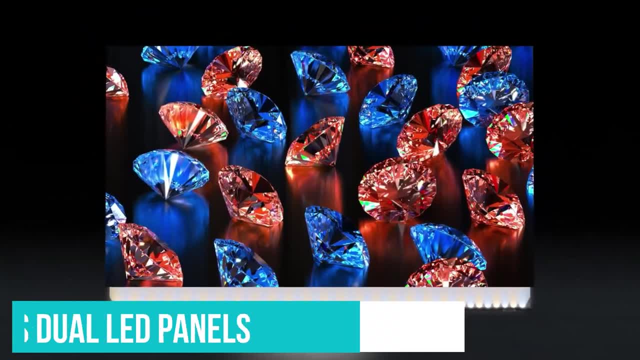 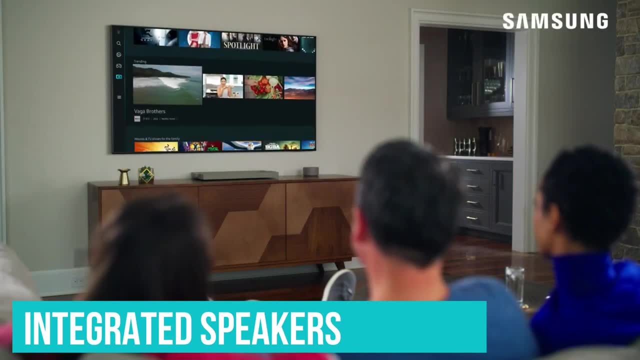 The QLED screen uses dual LED panels to create warm and cool colors simultaneously for a wider range of colors and more lifelike images. The integrated speakers give you excellent audio, but you can connect a Samsung soundbar and use a Q-Symphony feature. 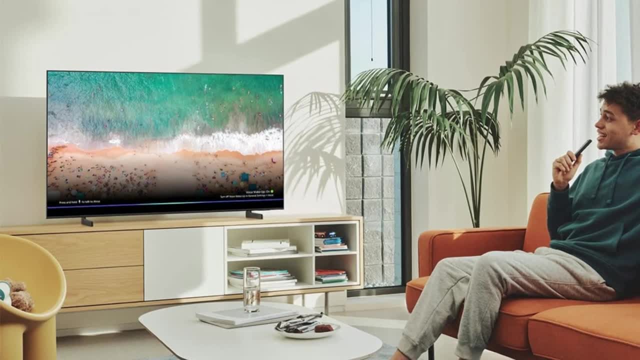 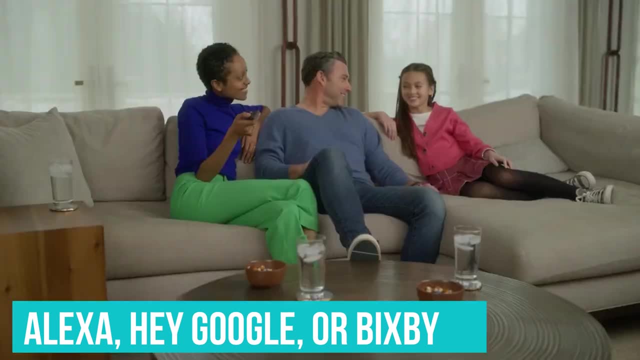 that allows sound to play through both the TV speakers and the soundbar for richer, room-filling audio without cranking up the volume. You can use Alexa, Hey, Google or Bixby for hands-free voice controls and even remotely connect the TV. 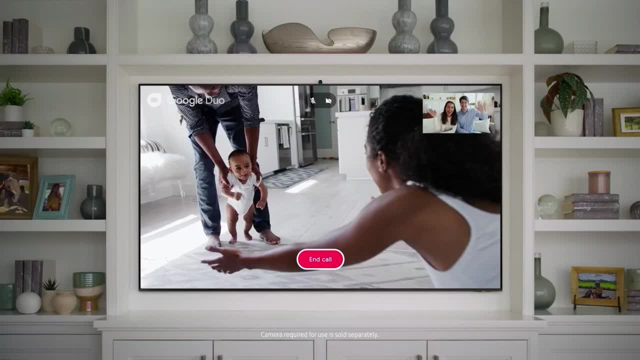 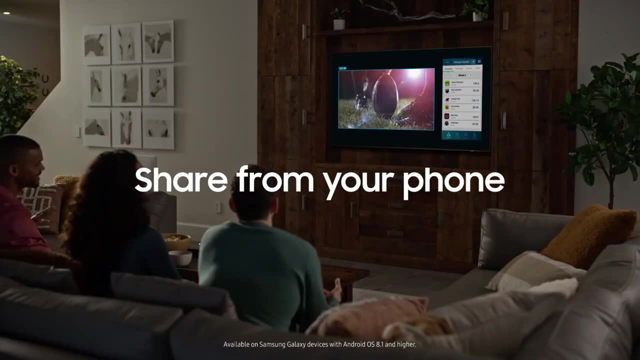 to your PC so you can stream games or work from the comfort of your couch. And if you want to make your home theater a little more eco-friendly, the remote for the Q60B has an integrated battery and mini solar panel for recharging. 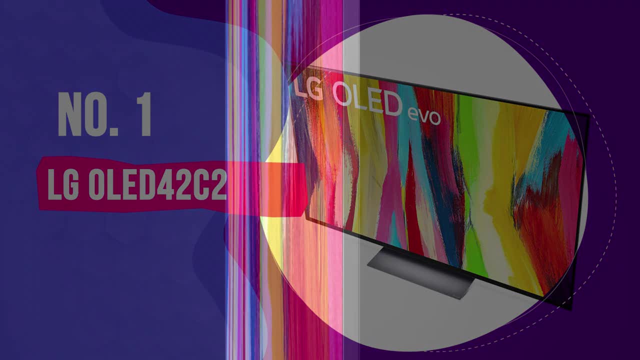 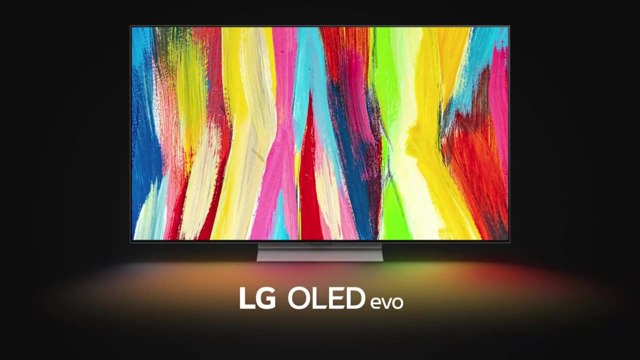 Number 1. LG OLED 42C2. The LG OLED 42C2 is the smallest size OLED screen And, despite Black Friday- now in the rearview mirror- it has retained its discounted price after the event, available for less than $1,000. 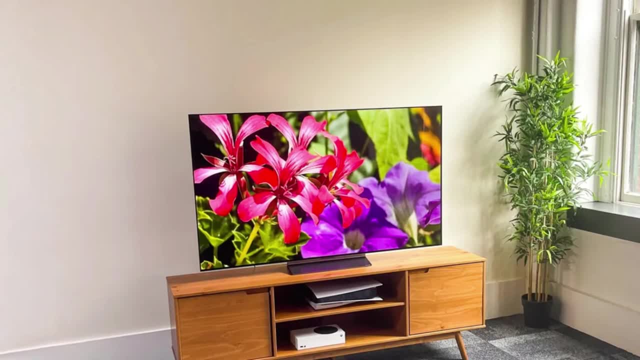 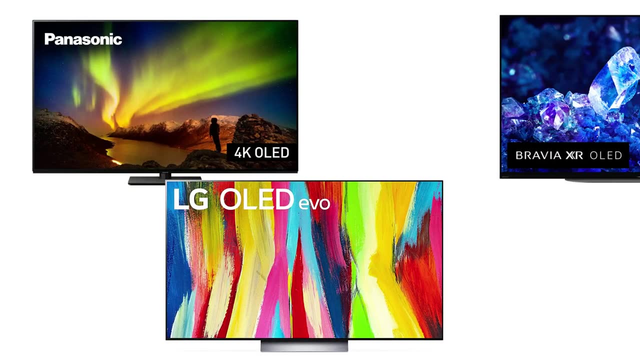 If you're looking to get a small OLED, now would be a great time to jump on the 42C2 model. It's cheaper than the closest rivals in the Panasonic LZ980 and Sony A90K And, while it arguably doesn't produce a better picture than either of these models, 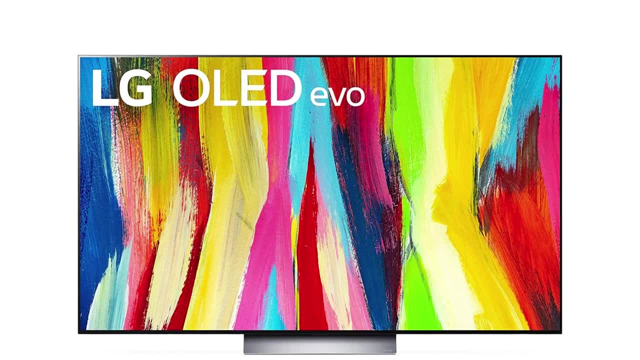 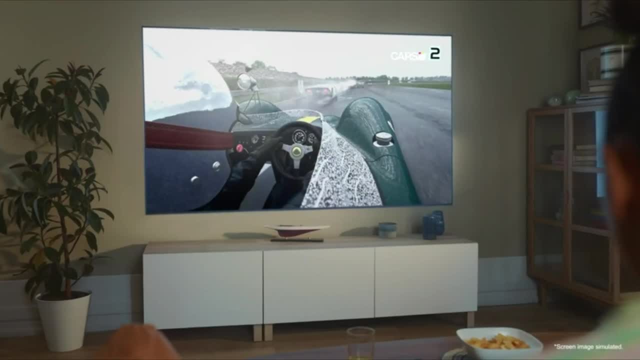 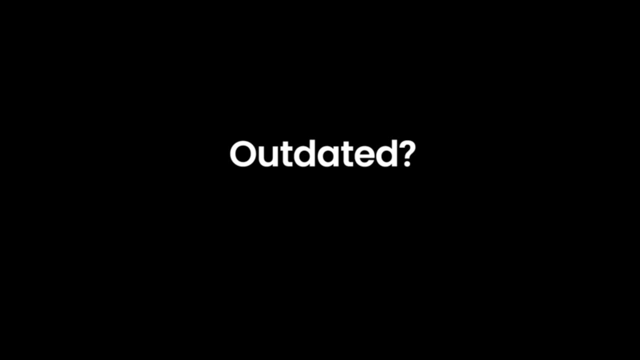 it does carry with it a range of features that we felt makes it an excellent choice for film fans, avid TV watchers and gamers. The 42-inch C2 is great size for bedroom gaming and comes with a bevy of high-end gaming features in VRR and 4K 120Hz, all of which are available across all the HDMI inputs. 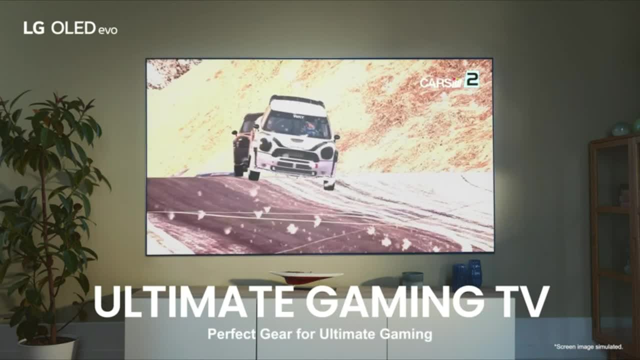 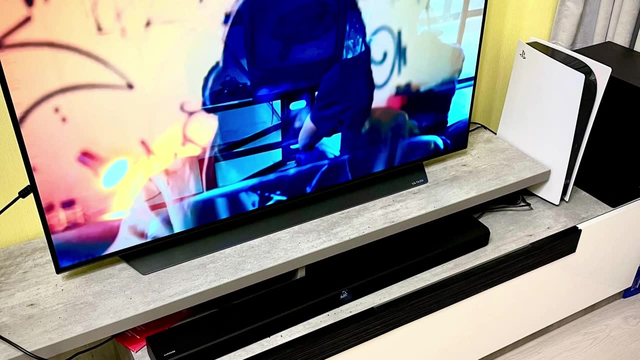 That means you won't be restricted by which input you plug your PC or games console. This also helps in adding a soundbar to this model, as you won't have to make a decision between whether to plug a console or soundbar in due to the eARC port. 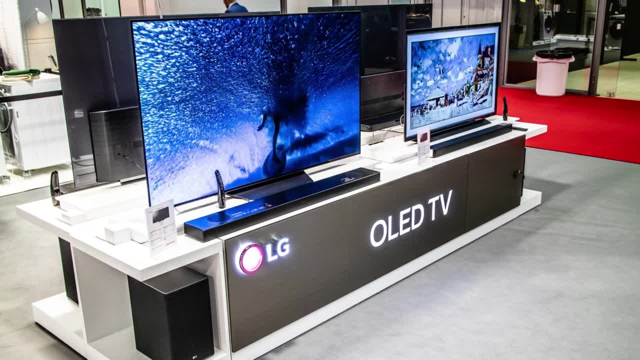 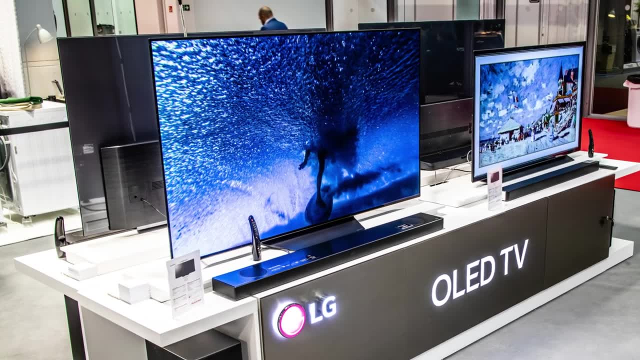 being shared with one of the gaming ports. Slotting a soundbar beneath this TV is tricky, given the feet don't elevate the screen that far off the table and most soundbars will block part of the screen. The design is one we feel is best suited. 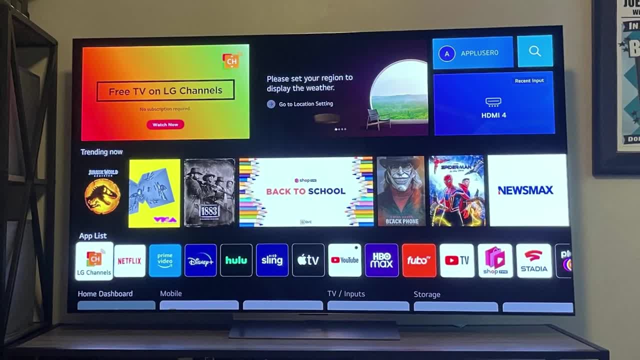 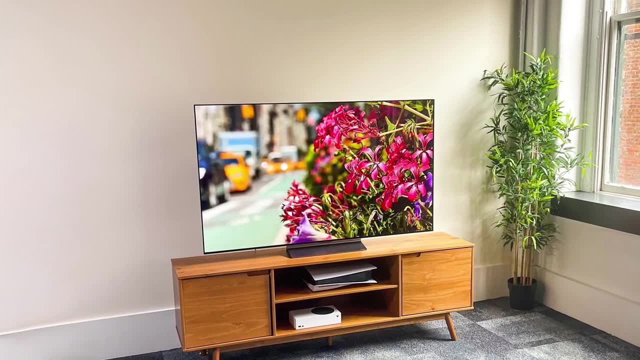 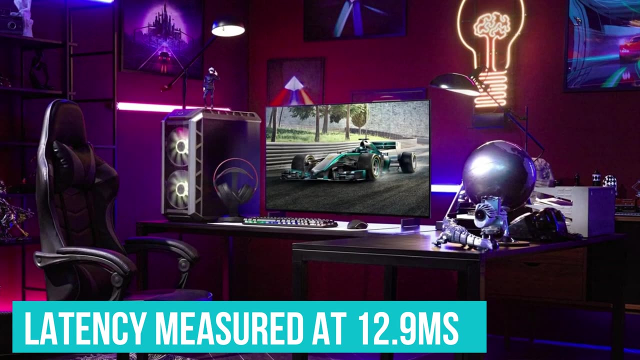 for being placed on a desktop flat surface rather than wall mounted. But irrespective of which orientation you decide to place the TV in, the connections are all side facing, which helps with plugging sources in. Back on the gaming front, and we measured latency measured at 12.9 ms, which is quicker than most TV brands. 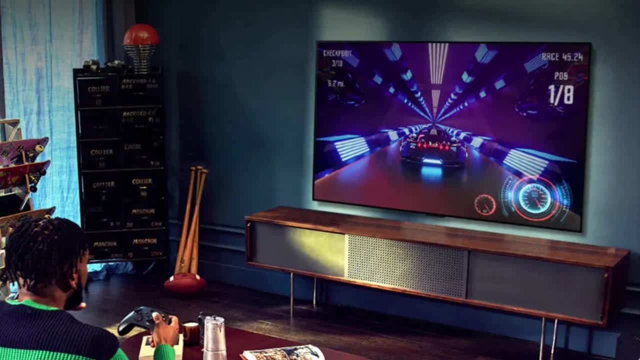 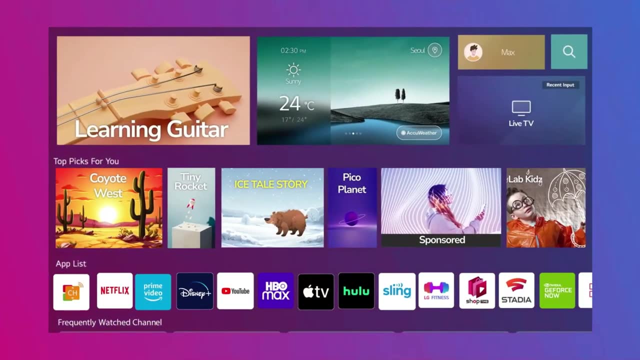 though not as fast as Samsung's TVs can be in general. Nevertheless, the VRR support, that figure can fall to almost zero in terms of lag. In terms of smarts, the OLED 42C2 has plenty, but avid TV fans will be impressed. 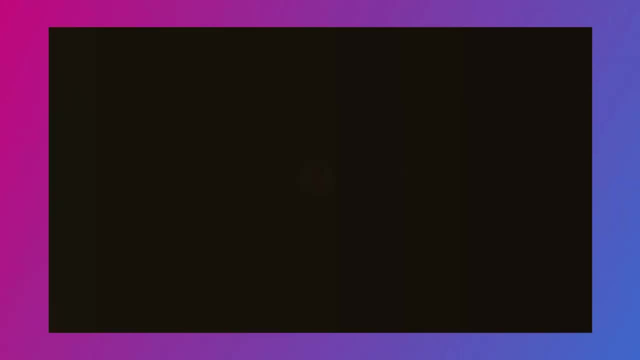 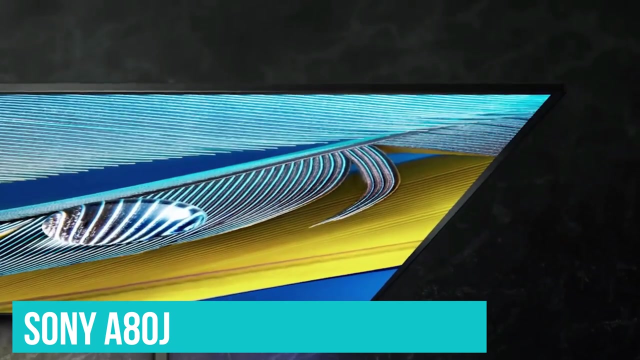 by the broad range of apps supported by WebOS, with all the major apps included, as well as Freeview Play that supports the likes of iPlayer and ITVX. Other than the Sony A80J, you won't find another TV on this list- delivers picture as good. 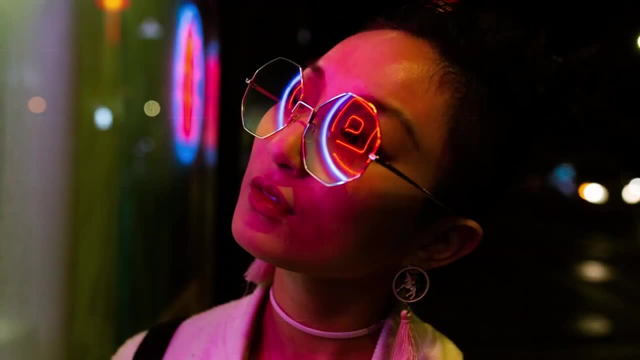 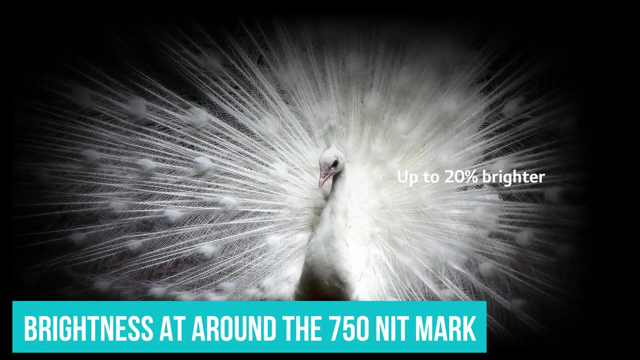 4K imagery was delivered in an impressively natural way, with a good range of colors as well as excellent levels of sharpness and detail. for its size, We measured brightness at around the 750 nitmark, which is plenty enough to act as a showcase for HDR content.